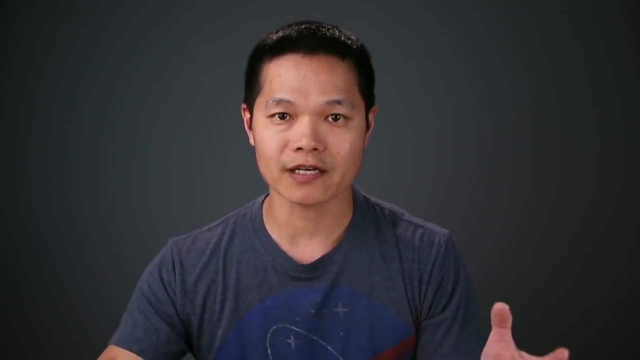 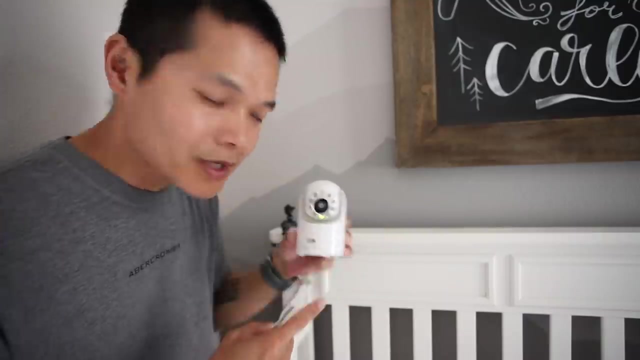 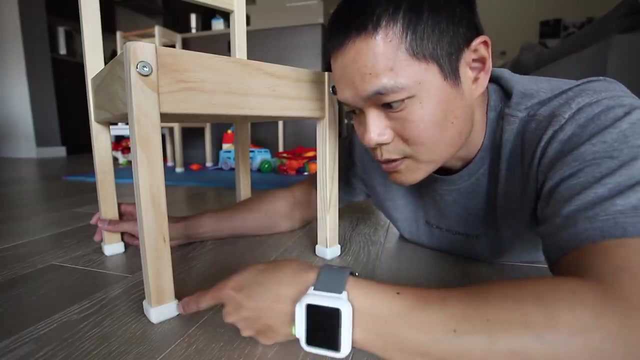 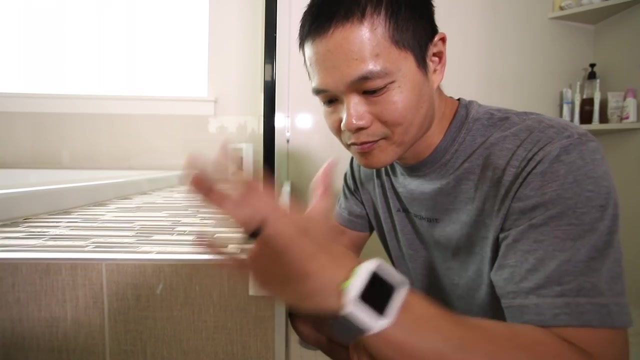 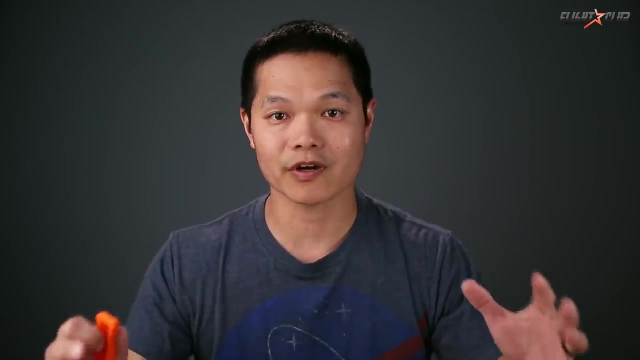 Even if you aren't into FPV drone racing, the skill of CAD and 3D printing is useful for everyday life. We use CAD to resolve everyday problems we have at home. The possibilities are endless. Boiled down to its essence: CAD or computer aided. 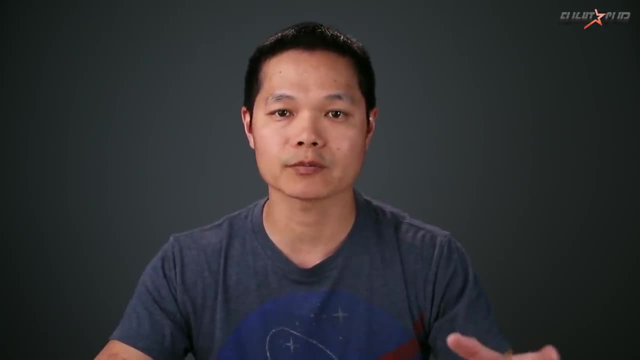 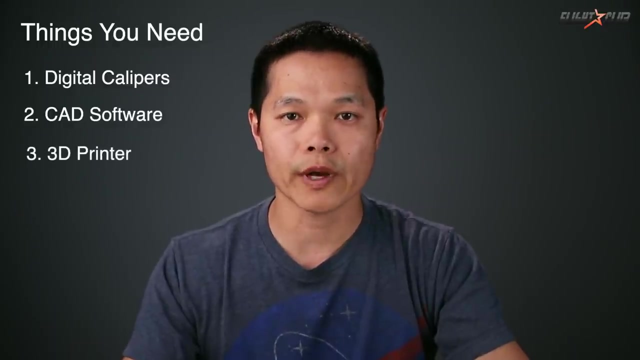 design is just adding or subtracting or, in CAD terms, extruding and cutting material away. First, there are three things. you need to turn your ideas into physical objects. you can use Digital calipers for getting measurements, CAD software to design your idea and a 3d printer or a way to turn your designs. 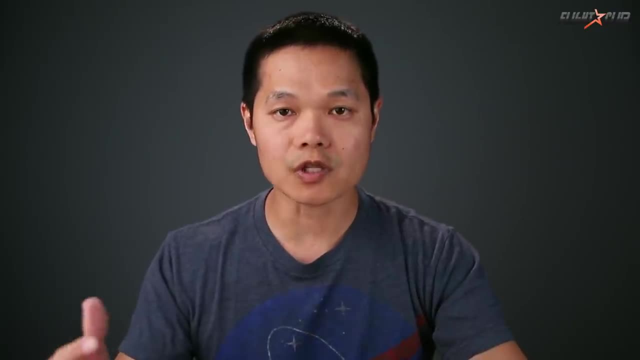 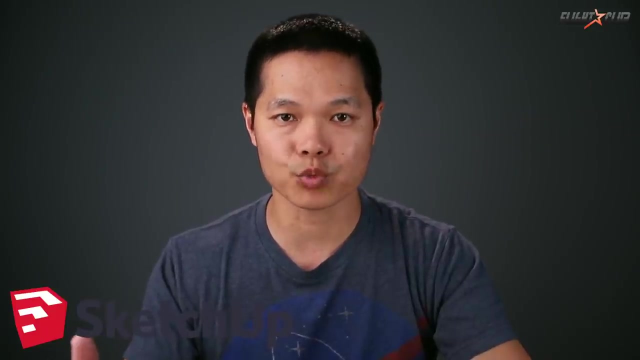 into a physical object. If you're just starting out, there's lots of free CAD software you can use online. Sketchup is a simple online CAD program that's pretty basic and it will let you export files that can be used by a 3d printer. 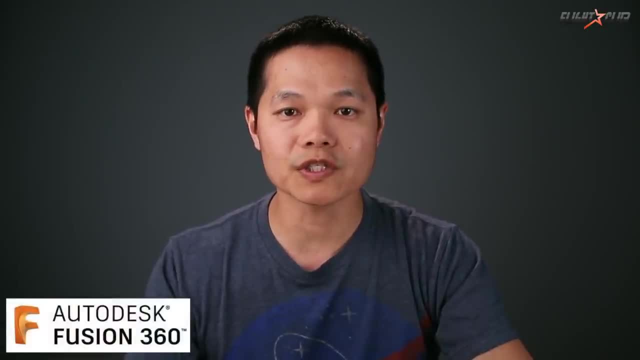 Then there's Fusion 360. If you're a student or teacher, you can sign up to use it for free. Fusion 360 is loaded with features and even has CAM or computer-aided manufacturing software to operate a CNC machine. If you're a total. 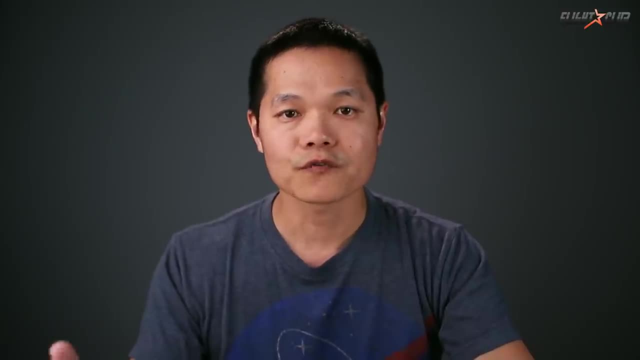 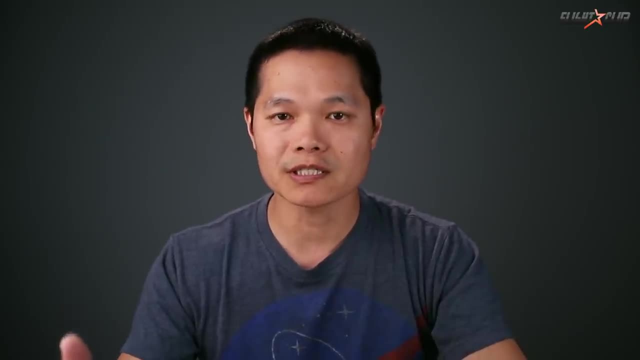 I won't get too deep into 3d printers in this video, but you can get a decent printer for under 200 bucks, and there's even companies online that will print items for you if you're not sure, if you want to get a 3d printer yet Once you. 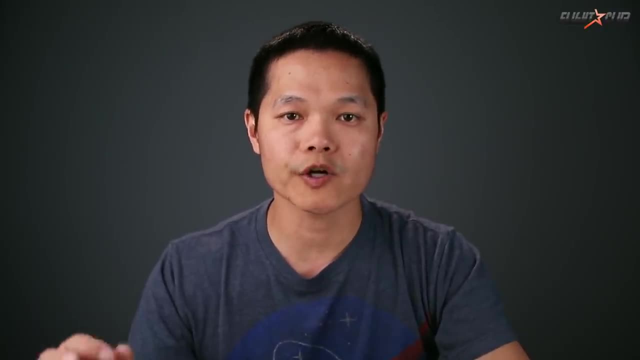 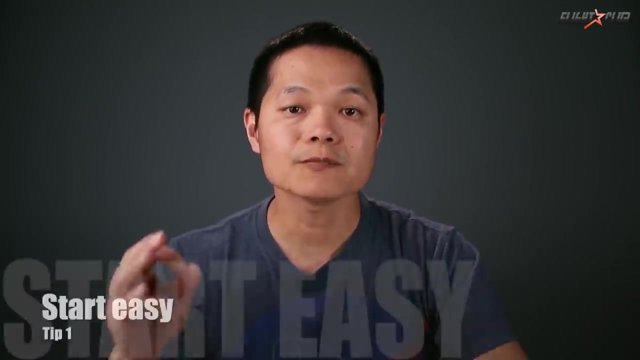 have an idea of what you want to make. you can start by planning on how to translate the idea in CAD so that it can be turned into a physical object by 3d printing. Here are a couple tips. Tip number 1. Start with something easy, Since this is a basic intro into CAD and 3d printing. 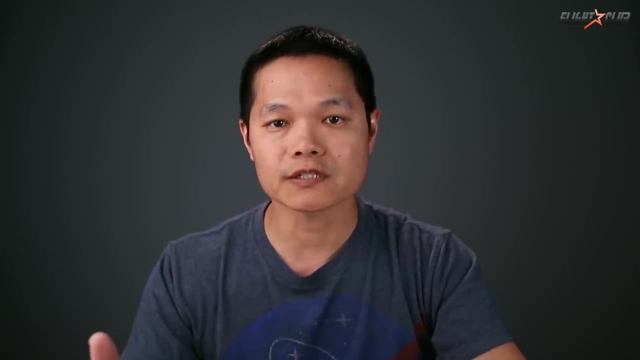 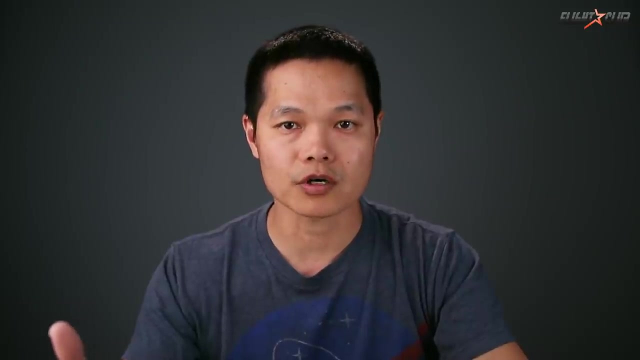 your design should have one flat side. The reason for this is 3D printing works by printing or oozing a melted filament or plastic layer by layer until you have a physical item. If the model doesn't have a flat side to start the print, it makes printing that object much harder. 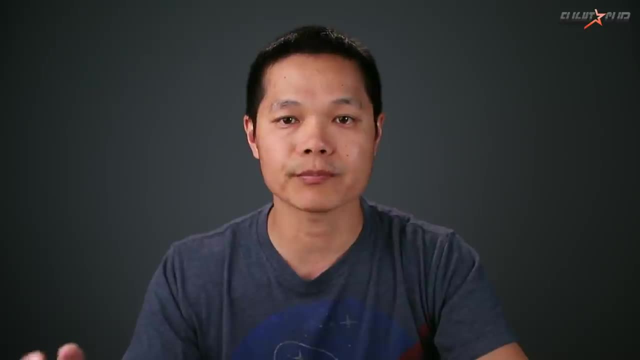 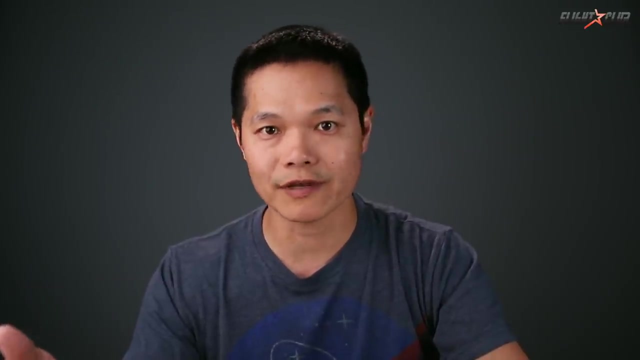 Without a flat side, you may have issues with the model sticking to the print bed. Tip number two: use metric measurements. This may be a personal preference, but I like to use millimeter measurements rather than inches. It's so much easier to say, for example, 10 millimeters rather than 0.39370079 inches. 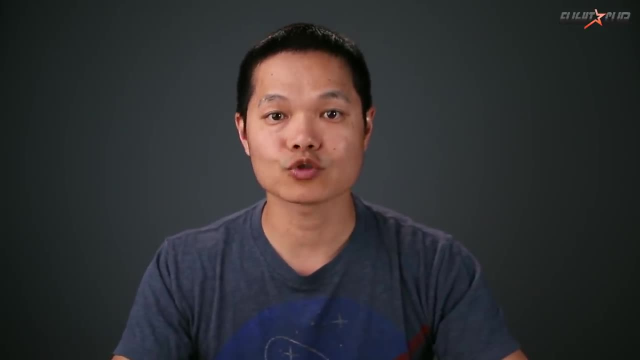 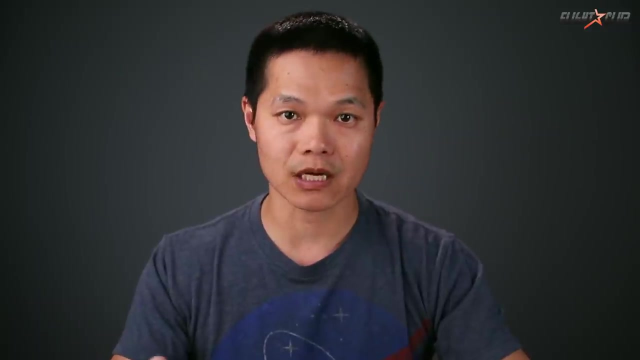 Let's get started. Since this is an intro into CAD tutorial, I'll just show you a simple overview of the basics of CAD. After this video, you should be able to design very basic items. Once you learn the basics, you'll learn more advanced aspects as you use CAD more and more. 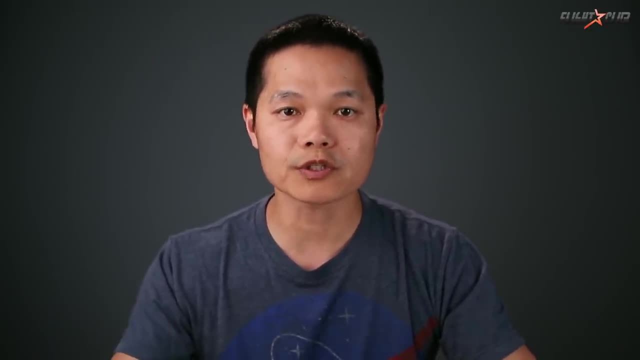 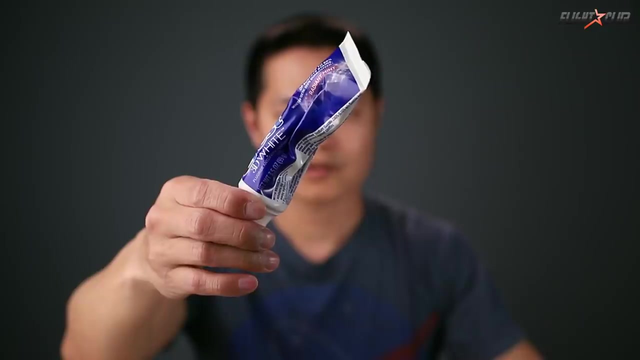 I learned CAD in SolidWorks, so that's what I'll be showing you. but the principles of CAD are are all the same in all the CAD software. In this tutorial I'll show you how to design this, to turn this. 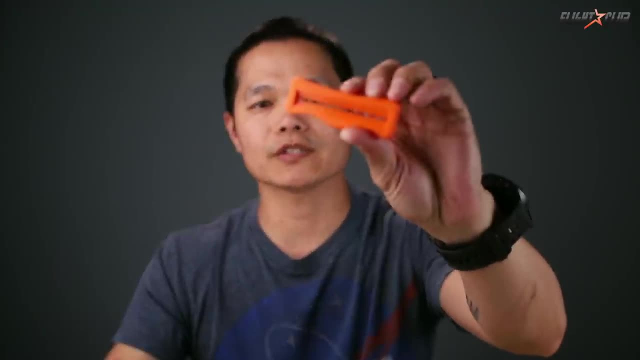 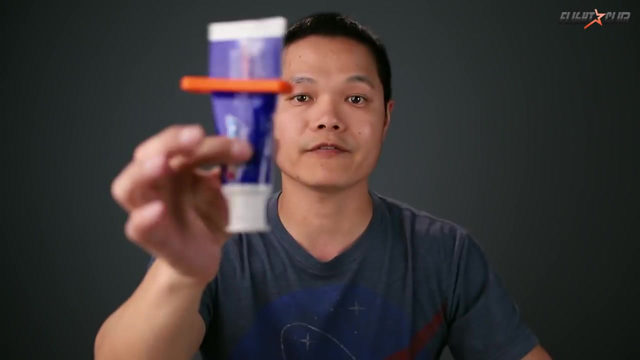 into this. This is just a simple gadget that squeezes the toothpaste from the back of the tube to the front of the tube, so you can squeeze from the center of the toothpaste tube every time. It's a very simple design and it's easier to design in CAD and easier to print. 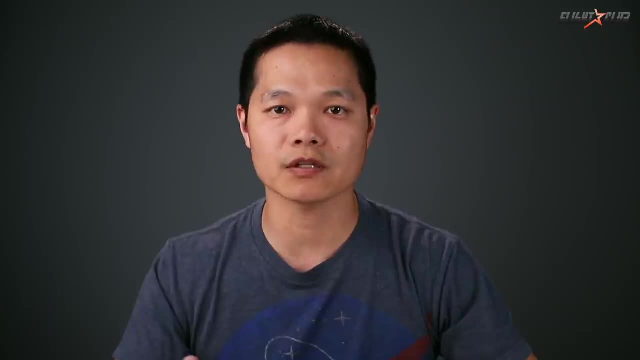 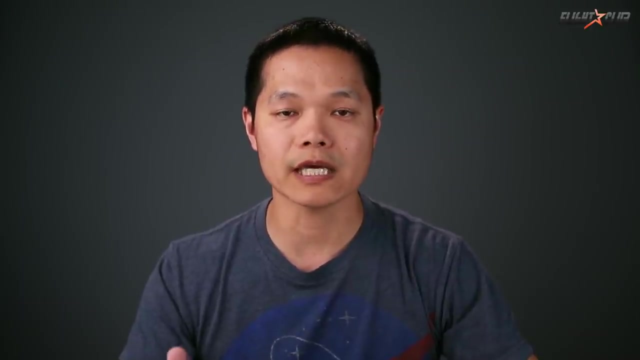 When you do a 3D design of physical objects, you have to think in three dimensions on the X, Y and Z axis. Normally the X and Y axis will be the width and height, and then the Z axis is the depth. 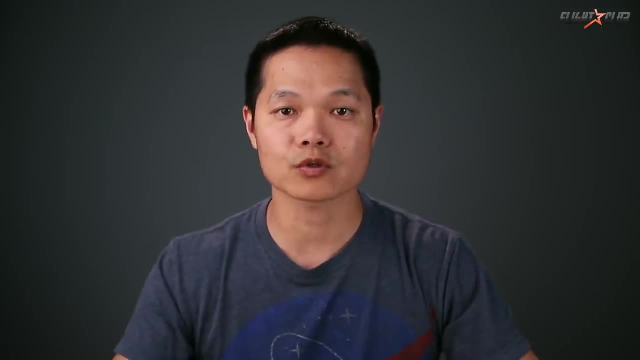 A drawing on a piece of paper would be a 2D or a two-dimensional drawing. You have the X which is left and right and then the Y which is up and down. This is a flat drawing. To make it 3D, you add the Z axis, which adds height to the drawing. 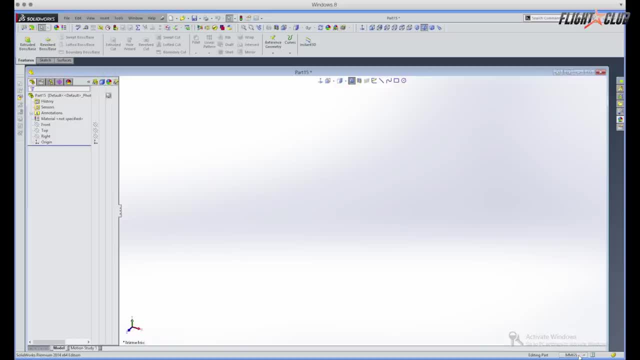 So the first thing you do before you start any drawing is you make sure you have the correct measurements of what you want to use. Right here, I'm using millimeters. If you want to use inch, select inch. So I'm going to use millimeters. 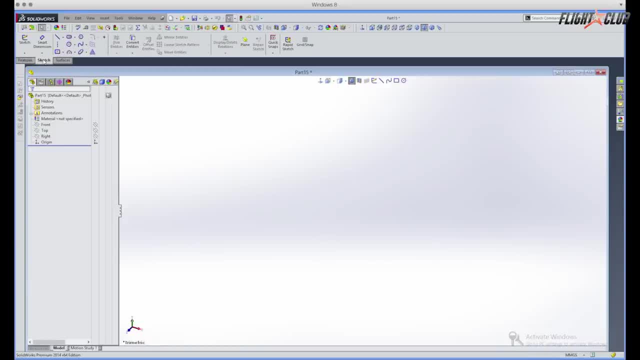 These are the two main tools that you'll be using in CAD. Sketches, which are drawings, and features are the extrude, or add, and cut, which is subtract. Like I said earlier, CAD is basically just adding or subtracting materials. 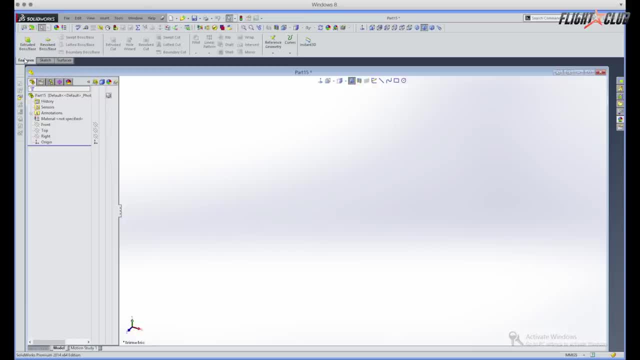 Just sketch, extrude or cut. sketch, extrude or cut, Sketch or extrude or cut until your model is done. It's really that simple. So in CAD, these three axes represent planes or sides that you can start your sketches on. 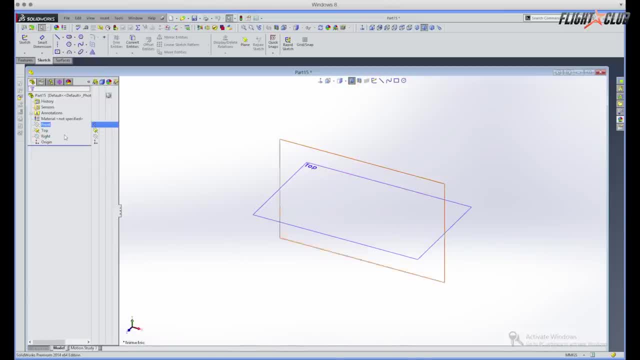 I usually start with the top plane because it's easiest to visualize. So to start, you might want to start with the top plane because it's easiest to visualize your sketch. just go ahead and select your top plane and then go up here and then create sketch. 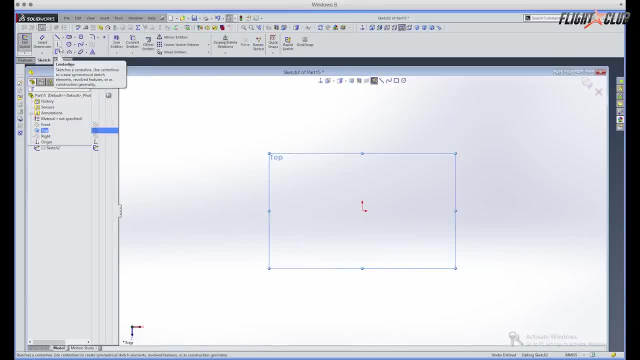 and then when you're in the sketch, you have all these tools that you can use to make your drawing. you got lines, you got squares, got slot circles, arcs, all these other different tools you can play with. so, for our example, we'll just use the rectangle tool and then start from the origin. 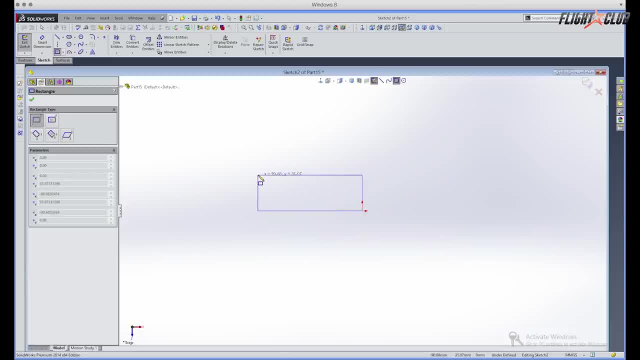 and then just draw out a rectangle, doesn't matter the the size right now. so once you've got the rectangle drawn, you're going to go up here and select dimensions and then you're just going to give this rectangle dimensions. so for our rectangle, for our toothpaste squeezer, we're 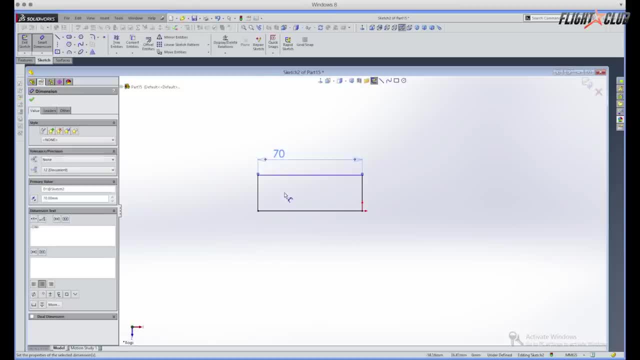 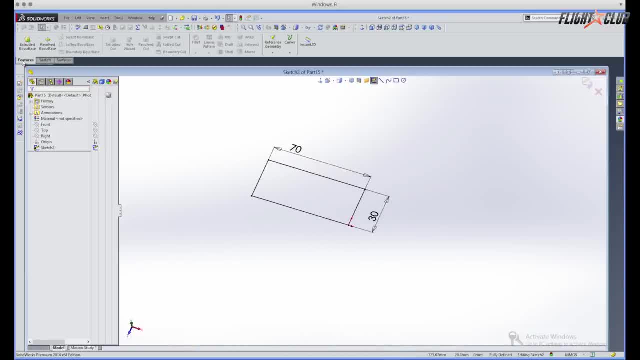 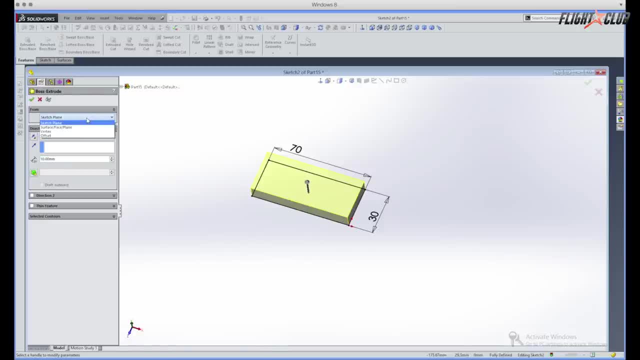 different parameters. you can start wherever you want to start the extrude. for this one i'm just going to start from the plane. and then here are different, more parameters of how much you want to extrude. so blind is just a set measurement of how much you want to extrude. so i'm just going to say 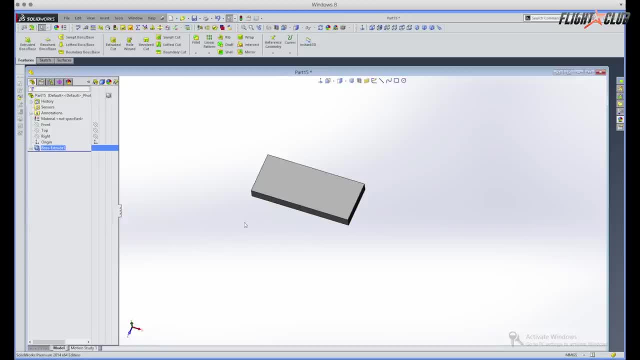 seven millimeters and then hit enter. so from our flat drawing over there, we extruded the drawing by um by adding seven millimeters of material. so next we'll make the slot that the toothpaste will get squeezed through. now, instead of using the um, the front right and top plane, we have a basic cube. 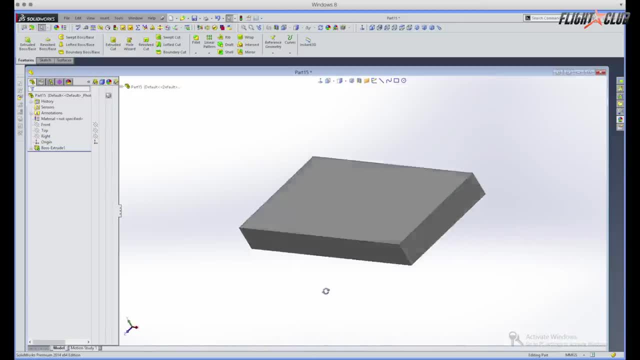 that we can pick any of these surfaces to start the sketch. so on this one, we're just going to pick the top surface and then go up here and hit sketch again, and then when you hit this normal two, it will make the the model flatten out to where you're just looking at that one side and then we're 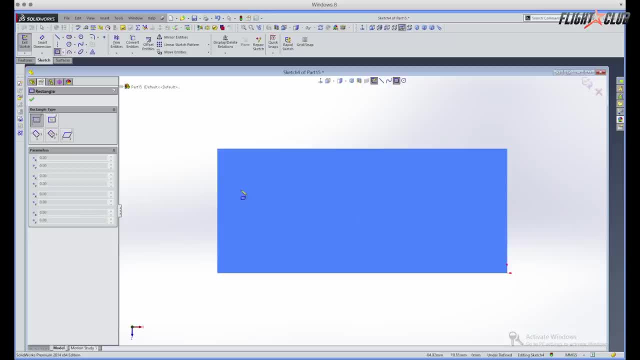 just going to draw a rectangle that we're going to cut out. so right here we'll just draw a random rectangle and then in cad, there are many ways to center a drawing. this is the one i like to use. if you pick this little center line thing, this is like a construction line. this doesn't draw anything. 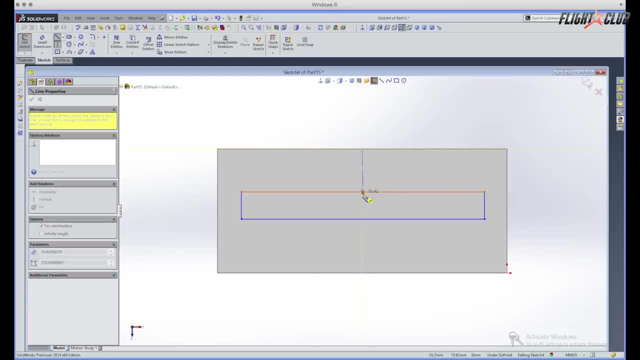 it's just kind of like for your own measurements. so i'm just going to pick this and then i'm going to select this and then, if you hover this, it'll show you the center of the line. so just click that and then, once you select this line, you can do different parameters. so i'm going to make this. 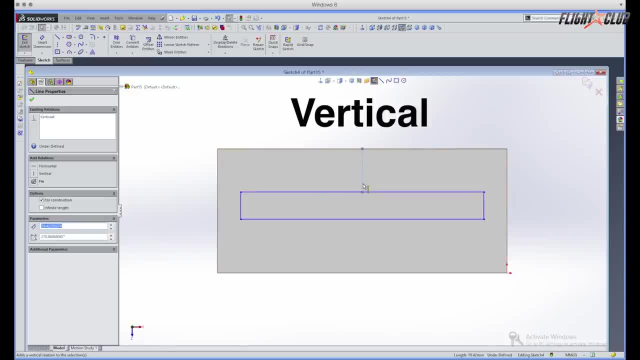 horizontal and this. this means this horizontal line will always center this line with this line, and then i'm just going to do another one for the side. so this is center here and then hover here and you'll see a little thingy pop up. click that and then select the line again and then click. 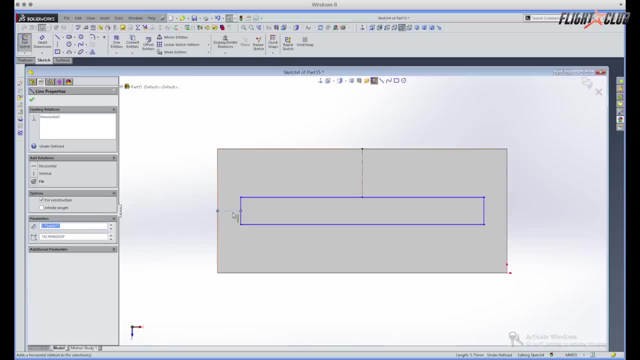 center. so this, these two lines, a vertical line and a horizontal line, will make sure that this square or this rectangle is always center with this shape. so once you have that, just go ahead and hit dimensions, and then you're just going to give this a dimension. we'll just say it is 65. 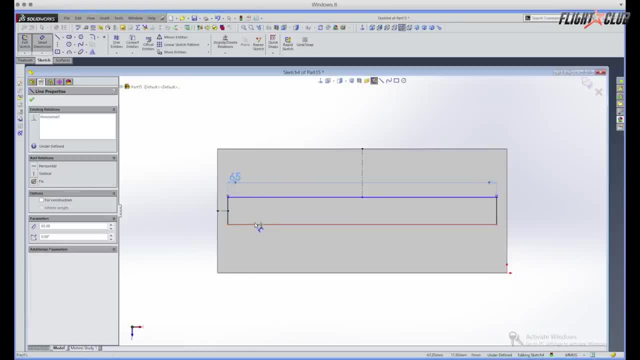 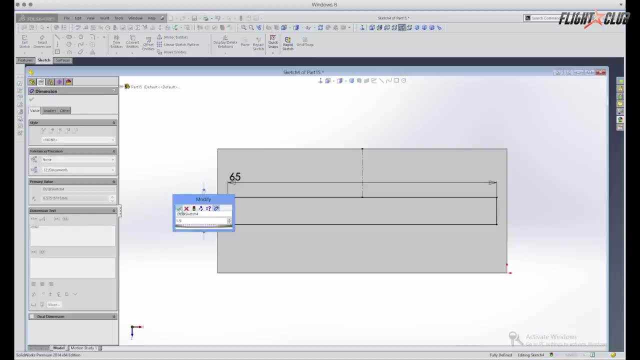 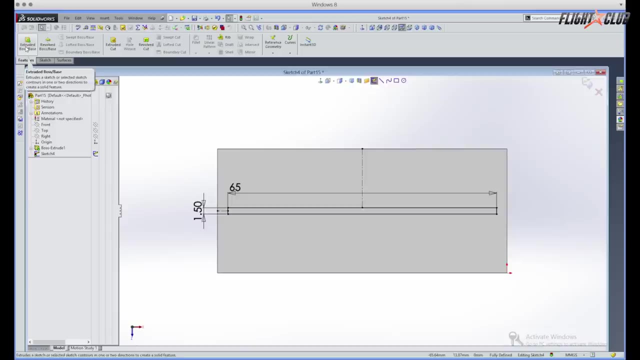 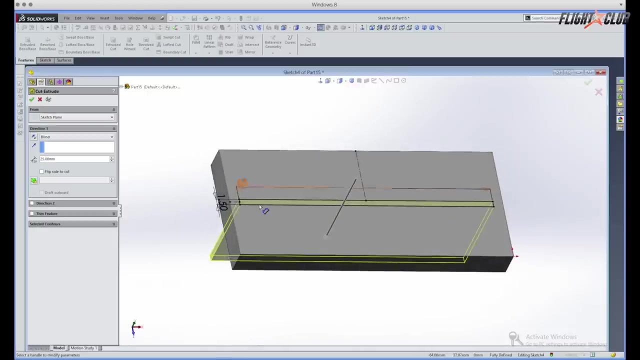 millimeters wide, and then we'll give it a depth, of say, 1.5. so now i want you have the sketch drawn, you can go up over to features and now, instead of extruding, we're going to cut. so cutting is just basically cutting away material. so on this one, i want the, the little slot. 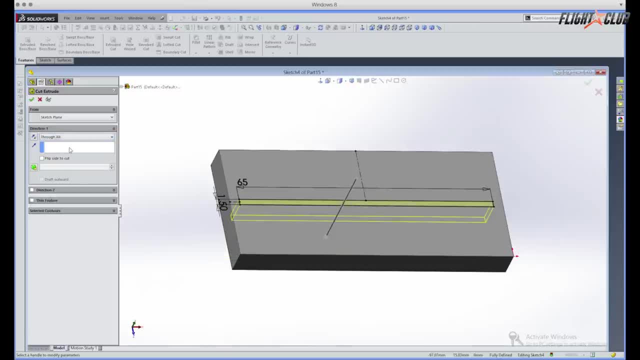 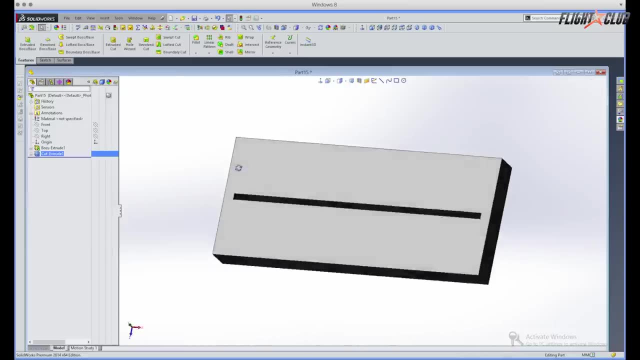 to go all the way through. so here i'm just going to go through all. if you hit through all this little sketch will cut through any part of your model. so let's go here now. you can see we have a basic little slot in our, our drawing. so drawing in cad is kind of like sculpting clay. start with. 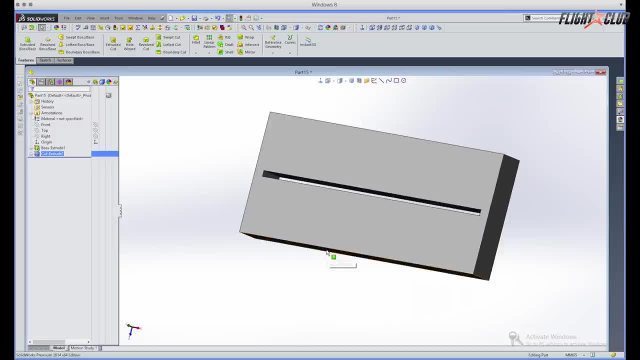 a really crude functional drawing like what we have here. then you just start adding details until you have a refined model. so essentially this is a working model of the toothpaste squeezer. we have a slot right here that the end of the toothpaste will be inserted and squeeze the toothpaste out. 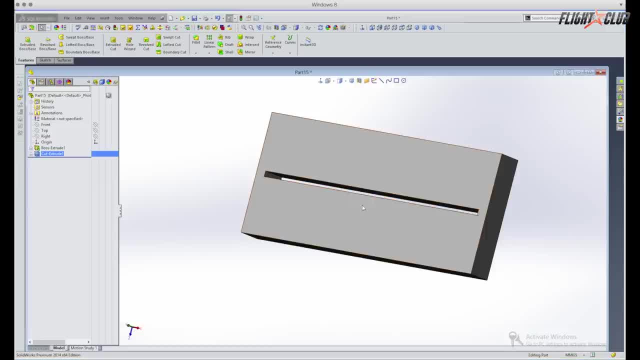 but we aren't done now. we add the small details that that improve the functionality and appearance. first we'll just add a slight curve to the ends of the toothpaste squeezer to make it a little bit easier to draw. so once again, i'm just going to start with the little slot and then i'm going to 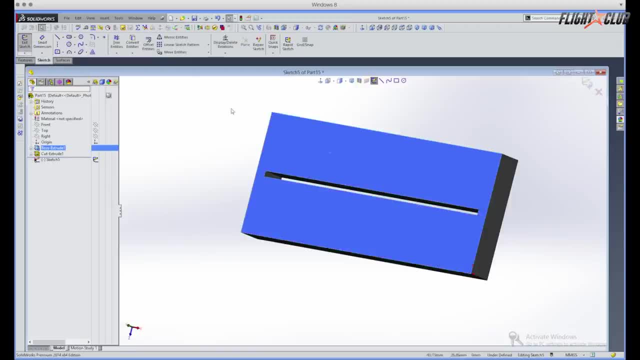 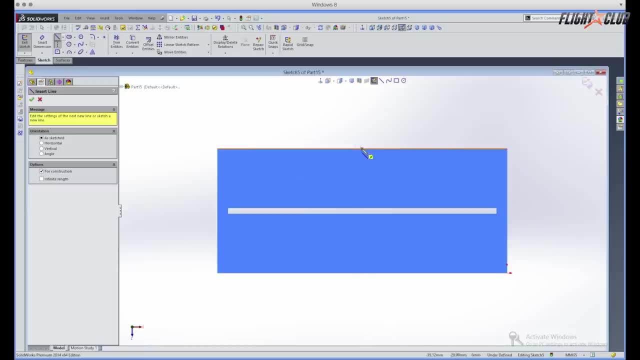 select this top face and then go to sketch, create sketch and then hit normal 2 so it's easier to draw. so for this one i'm going to draw a center line in this model- and i'll show you why later draw a center line and then when i do the drawing, i'm going to pick this little. 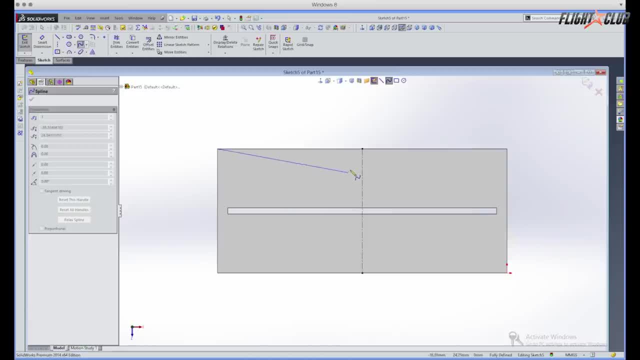 squiggly line. so this one you can kind of, you can tweak the line however you want. so i'm just going to do something like that, like that, and then i'm going to draw another line right here to the center and then from here i'll click mirror entity. so if you mirror entity, 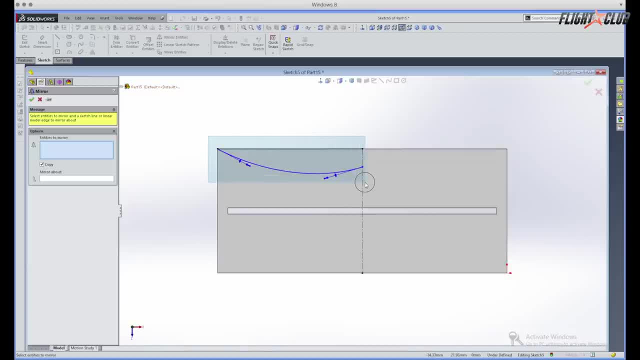 it's this: will you select what you want to copy and then you mirror, hit the center line and then whatever's on this side of the of the line will be copied over to this side select. so that's one part of our grip thingy and then the other half. i'll just draw a simple. 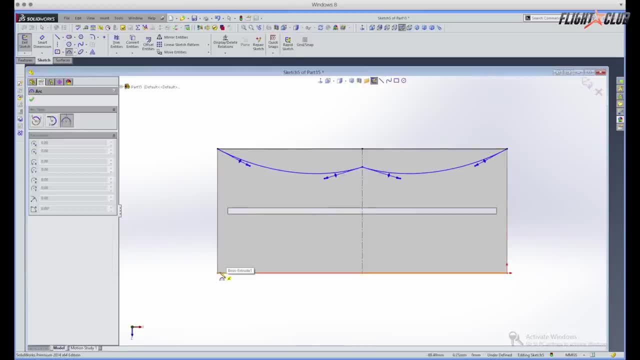 line over here and then go draw a little arc just to give it a little bit of a curve. all right, so we have our drawing on the top and bottom. now we can go to features and go extrude, cut, and then i'm going to cut away this part of the drawing. so i'm going to go through all select. 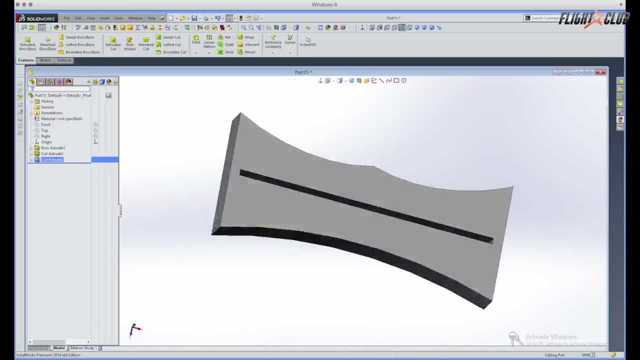 okay, we just gave our little toothpaste squeezer a little bit of a grip for your fingers. next, since this little slot is kind of crude, we're just going to make it a little bit easier for the toothpaste to be fed through. so for that we're. 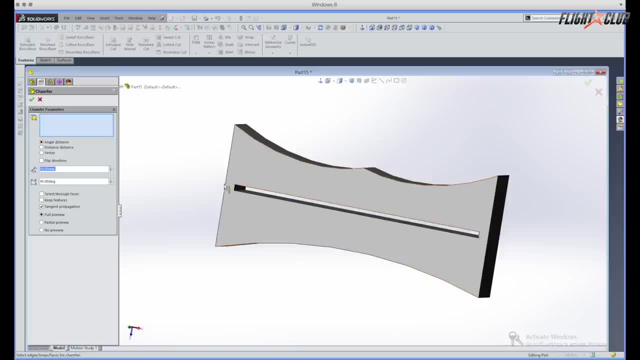 just going to use the chamfer tool. the chamfer tool cuts edges to whatever specifications you give it. so we're just going to give it a um, a distance of, just say, five millimeters and then we'll keep the 45 degree. so when i hit this little edge right here it's going to mean it's going to have kind of a generally now for you to know if i'm cutting theido or fixing the compiled. but you can see here you'll notice shape style kind of stops going through each of theодic and curve parts like that, and so you can see a. 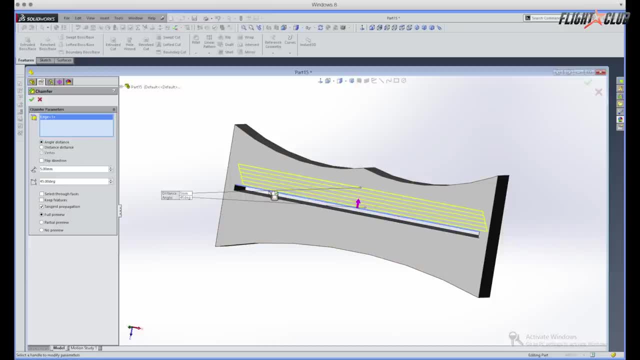 littleub. we'll kind of check. the Top rechtar along the top right is how much grid this piece right here if you don't know degrees. So when I hit this little edge right here it's going to cut 5 millimeters at 45 degrees. 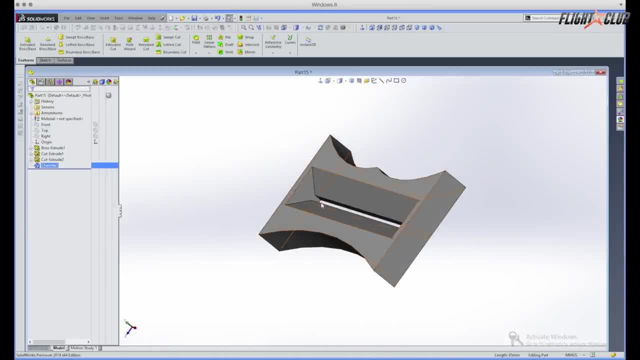 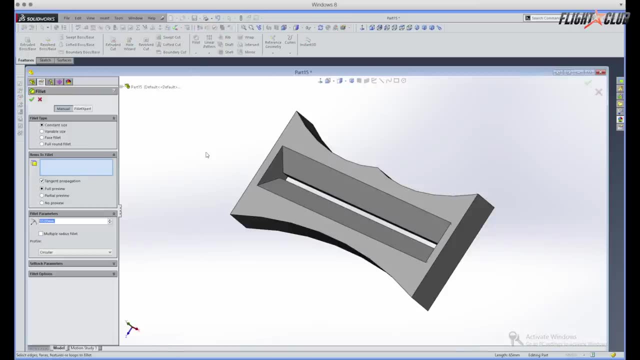 So you can kind of see there: Hit enter. Now you see we have a little slot that the toothpaste will be easier to feed through. Now, last is my favorite tool. You're just going to use the fillet tool. The fillet tool just rounds out edges and just makes things look more pretty. We'll just 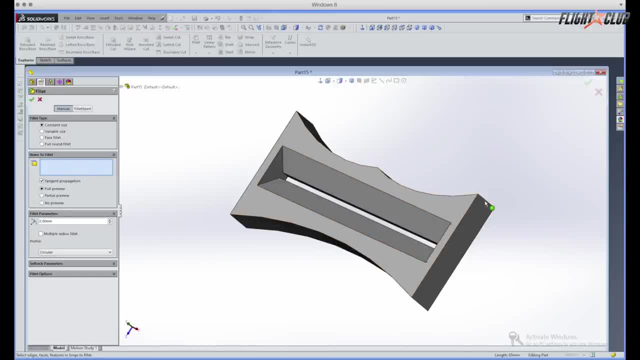 give it a parameter of 2 millimeters, and then we're just going to start rounding out all these little edges to make it a little bit more round. We'll do this edge, this edge, And we'll give this edge and this edge a little bit of a roundness too, Once you hit that. 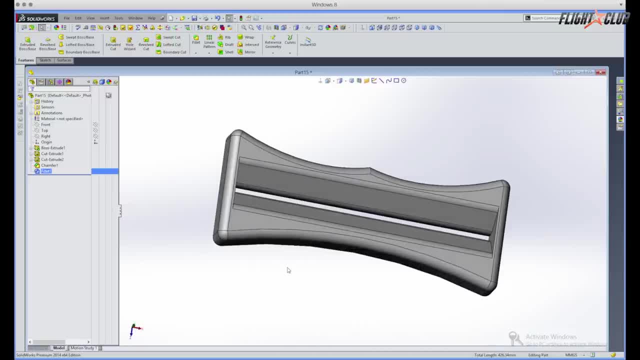 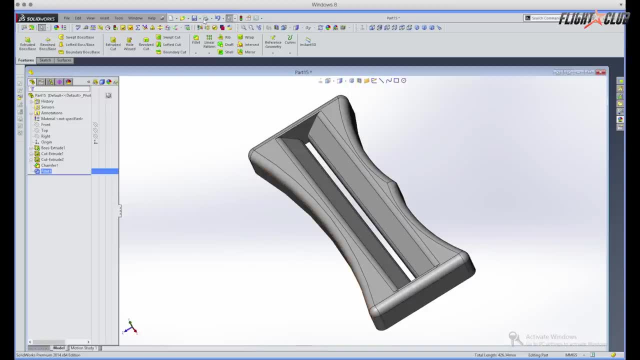 now you can see it looks much prettier than that blocky thing we have. At this point we're pretty much done with the design of our toothpaste squeezer. So when you're done with the design you just go up here and you save. 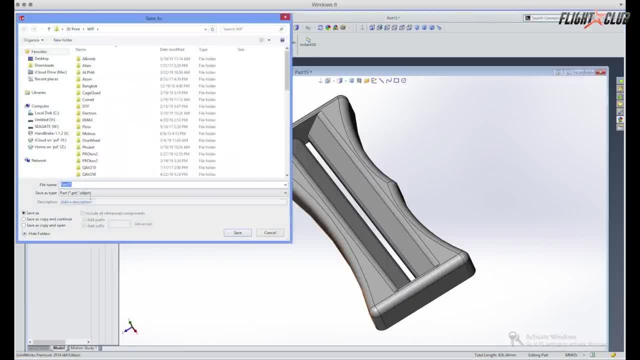 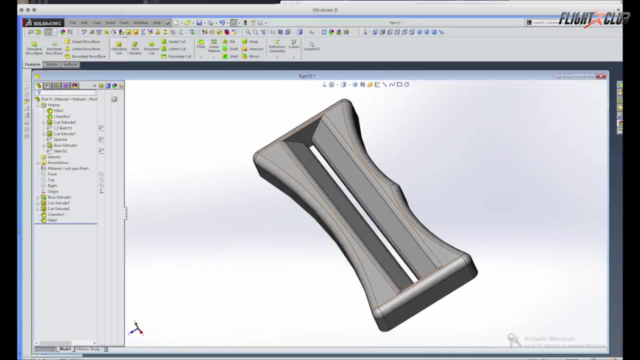 This model as a STL, So we're just going to bring it over here and then call it toothpaste squeezer. And then you want to make sure you save this as a STL file, because the STL file is the file that's used for 3D printing. So once you have your STL file now, you can put the file into a. 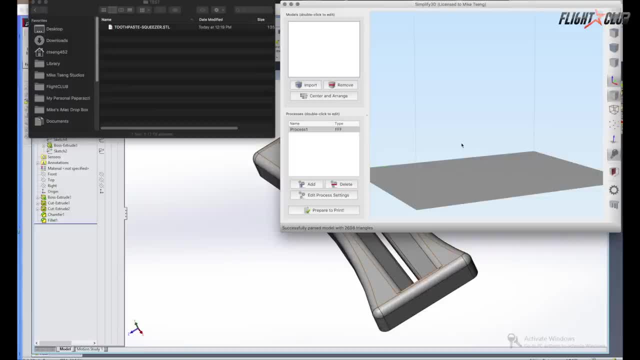 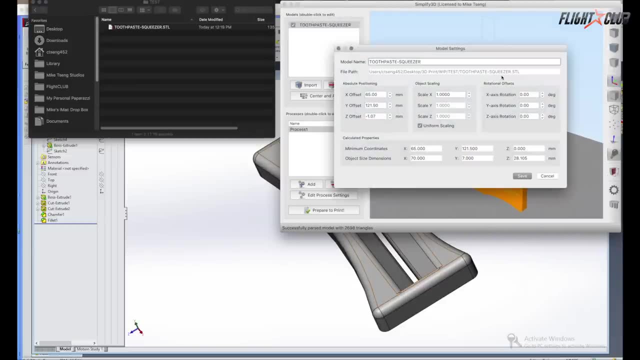 slicer. A slicer is basically a program that tells the 3D printer how to print this file. So you just want to make sure that your file, your flat side of your, your file, is facing down. So we're just going to rotate it. 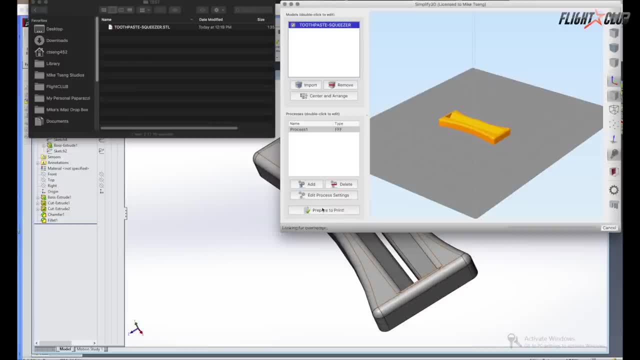 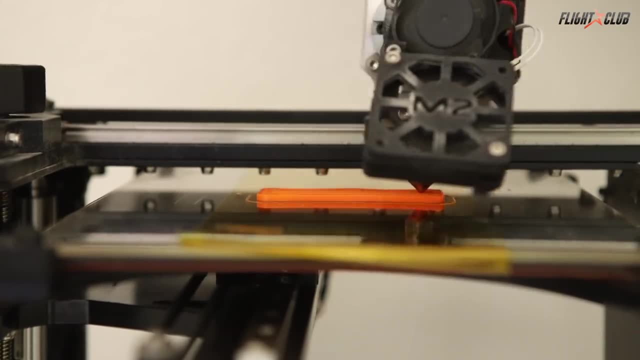 And then from there you're ready to start your print: Hit, print and print. I know this is a ridiculously short tutorial, but it should demystify CAD enough for you to get in there and start designing basic items. Once you learn the basics, you can go on and learn the.